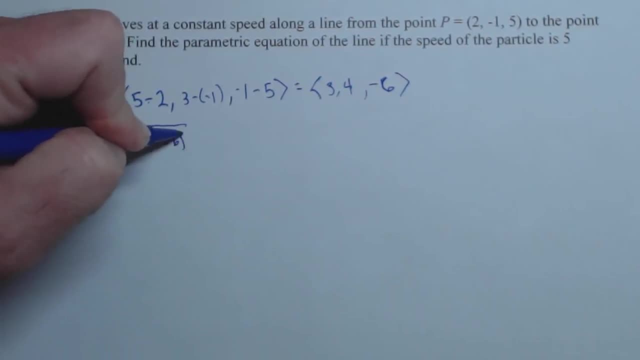 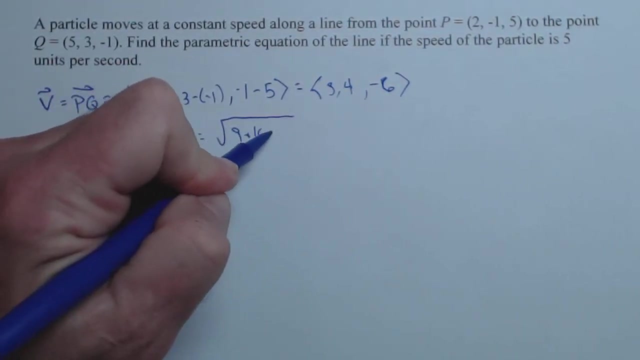 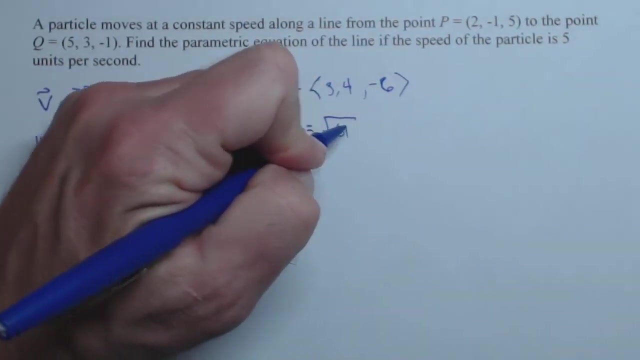 components. So we are going to have the square root of nine plus 16 plus 36, which let's just keep it as a square root. We'll keep it nice and exact. We can always change it at the end. So square root of 61.. Now I wanted the magnitude of the velocity to be five. 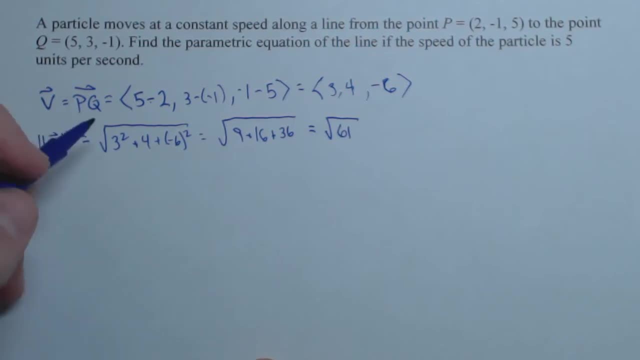 So what I'm going to do is I'm going to make the velocity vector a unit vector. So this new vector- let's call it w- is going to be 5 over square root of 61 times our original pq vector. Now let's talk about this for just a sec. 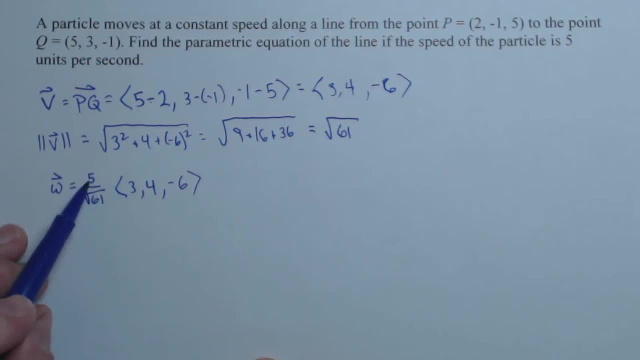 We're dividing by the magnitude, That makes it a unit vector. Then multiplying by 5 guarantees us that we have a magnitude of 5.. So we know that the magnitude of this vector w is 5.. So, basically, what we're going to do now is the antiderivative of this. 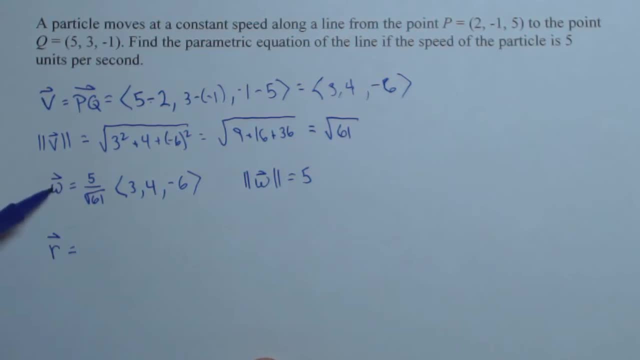 So when I'm going to find r, the position vector, it's the antiderivative of w, which would be some initial position x0, y0, z0.. Plus, basically these are all constants. so I would just add in a t. 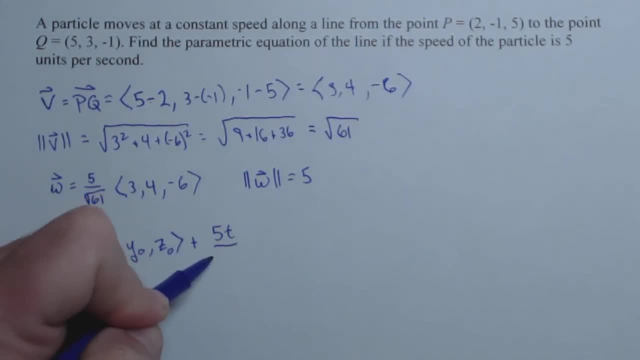 and I'm just going to add it out front: 5t over square root of 61 times 3, 4, negative 6.. Now we haven't really said when we're going to be at what point, so probably the easiest is just to say: how about at? t equals 0,. let's be at point p. 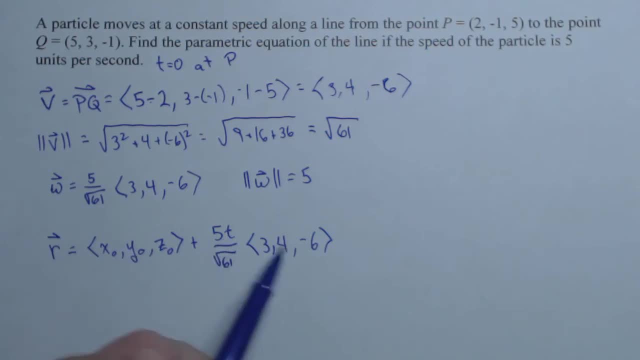 Cough, cough, cough, Because what that does if t is 0, this all cancels out, and so my initial position is actually just the point p, So that'll allow my vector r to be 2 minus 1, 5,. 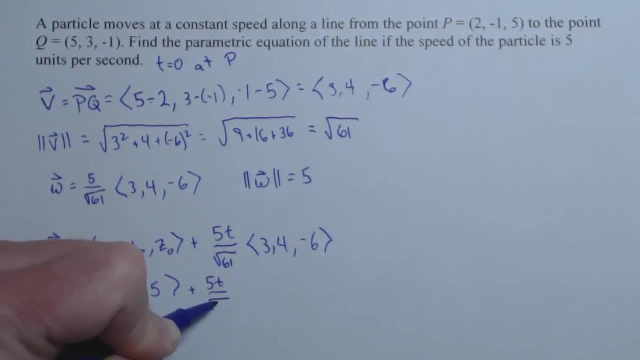 plus 5t, over square root of 61, times the vector 3, 4, negative 6.. So this will meet all of our requirements. Now we could write this as: x of t, y of t, z of t. 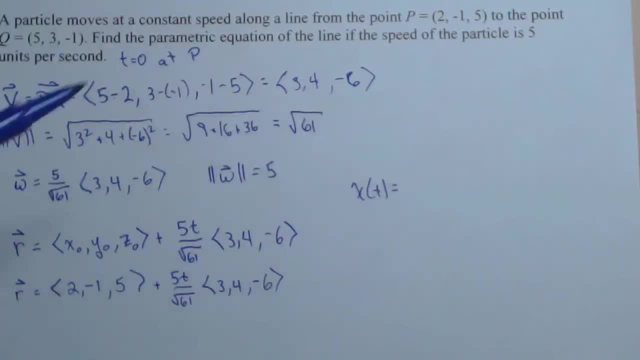 And so what that would look like. let's just put them over here so that we have them. x of t would be 2 plus 5t over rad 61 times 3.. So maybe we'd write it as 15t over square root of 61.. 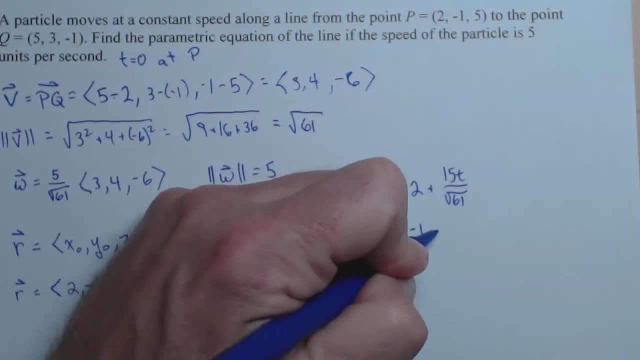 y of t is going to be starting at negative 1.. And so 4 times 5 is 20.. So we're going to have 20t over square root of 61.. And finally we've got z of t, which is starting at 5.. 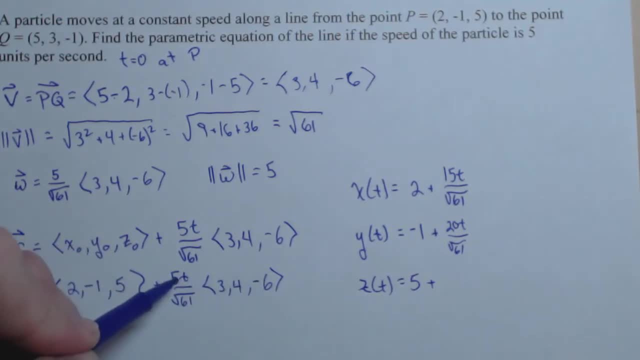 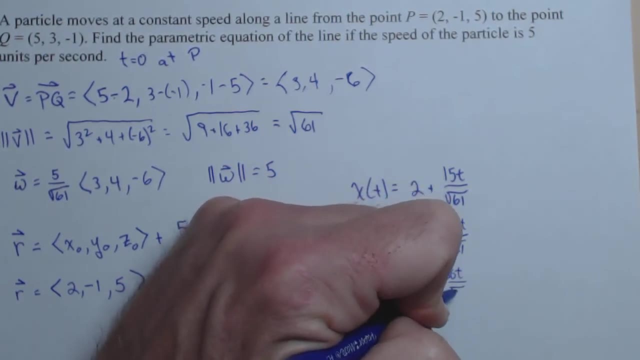 And going to end at negative 6 times 5, which is negative 30t over square root of 61.. And if we wanted, we could have just made it 5 minus. So let's just do that: 5 minus 30t over square root of 61.. 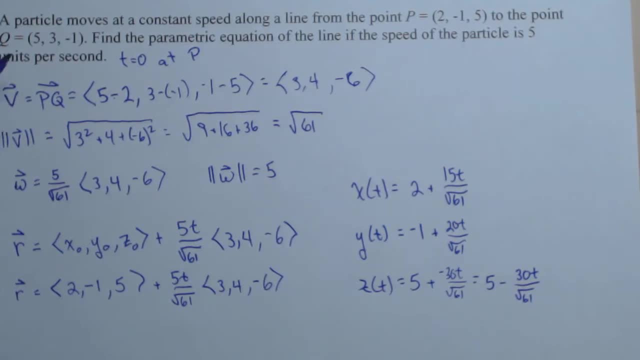 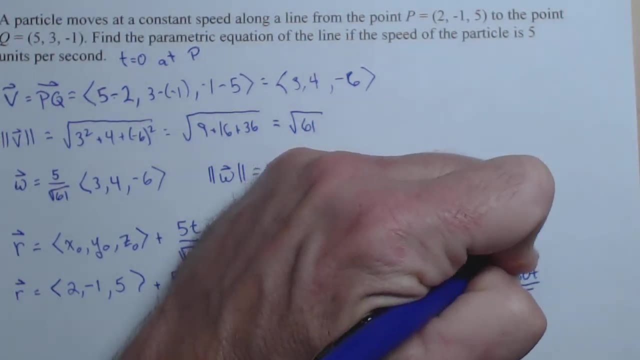 Now let's make this thing end at point Q, Because we do need to give a t range for this. Well, we know that we're starting at 0. And we can see that pretty clearly, because 0 is going to cancel all those out. 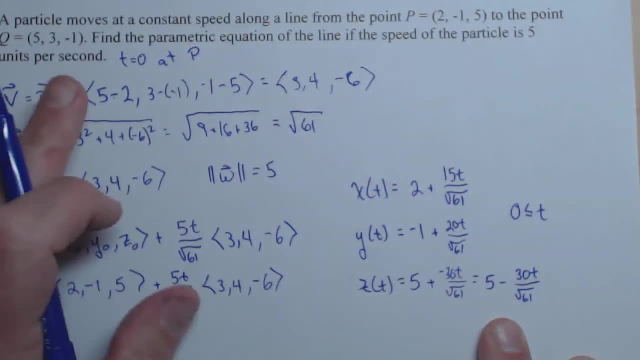 which would put us at 2, negative 1, 5, which is point P. We want it to end at Q: 5, 3, negative 1.. Well, remember what we did to our vector PQ in order to make it have a magnitude of 5.. 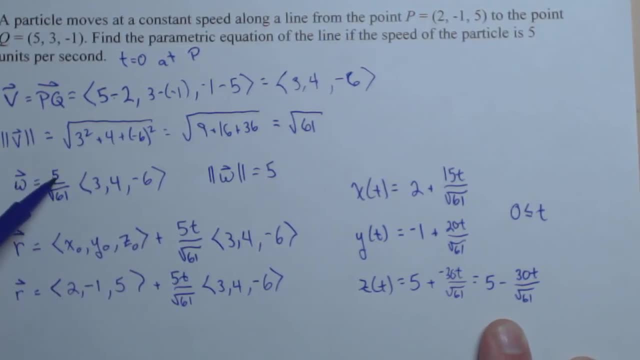 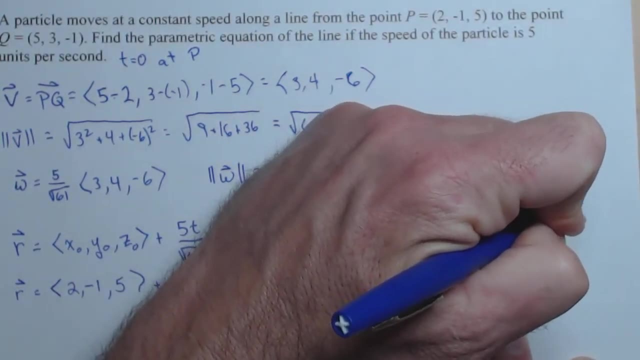 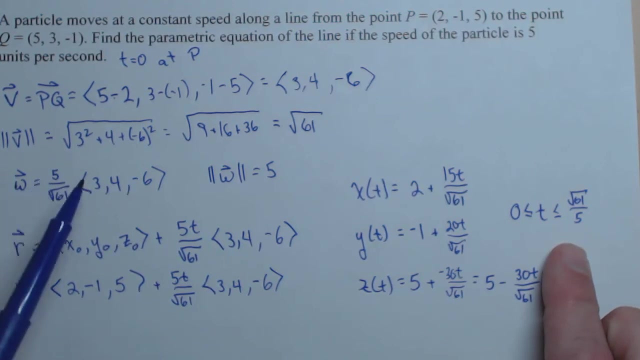 We multiplied by 5 over rad 61. So to undo that, we just have to multiply by the reciprocal, So square root, of 61 over 5, we'll make sure that we end at point Q. If we don't see that right away, imagine multiplying, for instance, x of t by rad 61 over 5.. 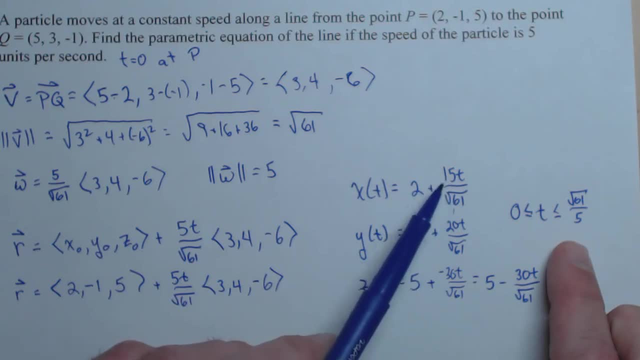 The rad 61s would cancel, We'd have 15 over 5, which is 3.. 2 plus 3 is going to end us at 5. And it's going to be the same for the other two coordinates.